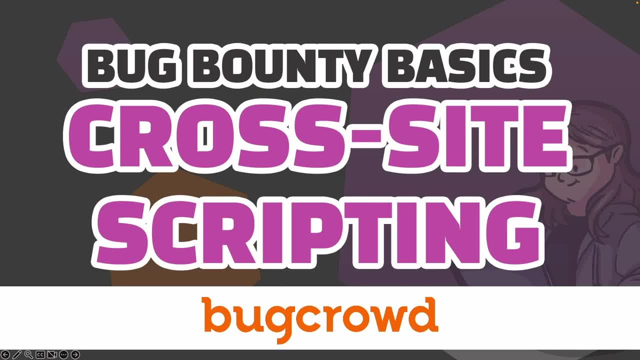 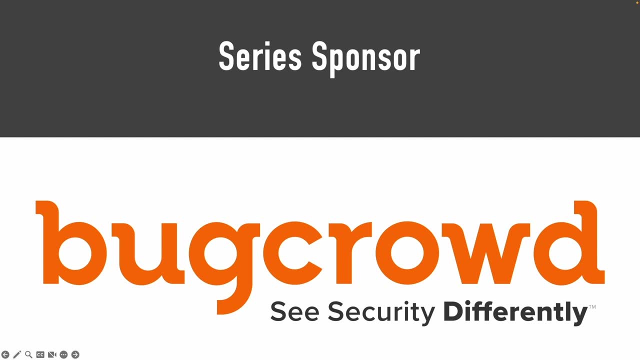 outside of really specific questions, targets or really specific technology stacks, but cross-site scripting is still really, really common. it's one of the most common security vulnerabilities, so we're going to talk about it once again. this entire series would not be possible unless we could get support from. 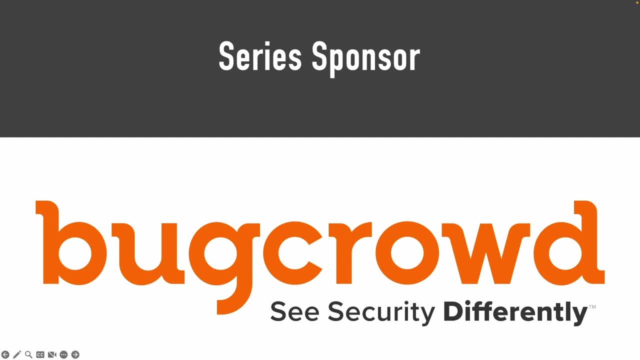 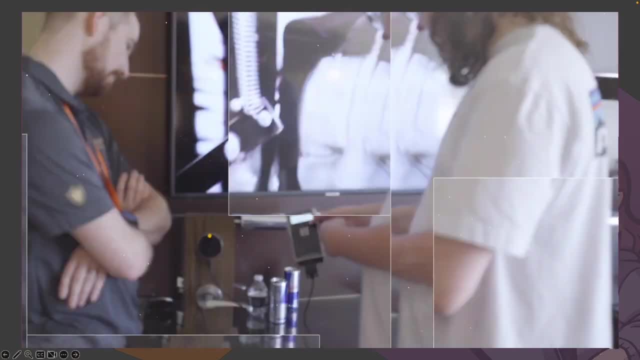 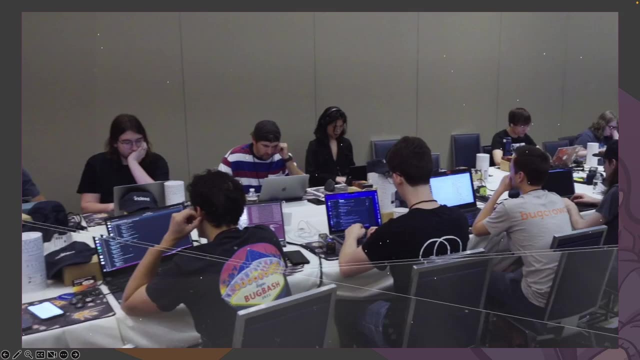 sponsors, and our sponsor for the whole series is bug crowd. bug crowd is the best place to start hacking with a wide range of public and private programs, from apis to desktop applications and everything in between. not yet ready to jump into a public program, fill out your platform cv and sign. 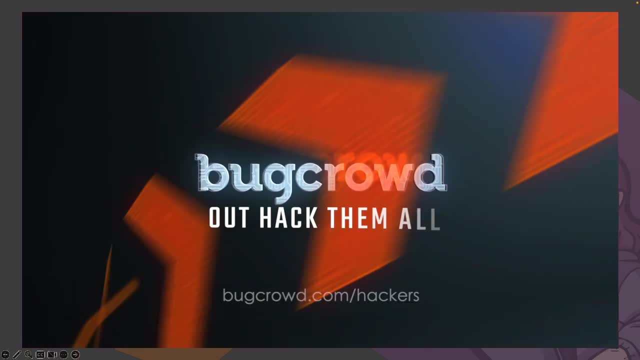 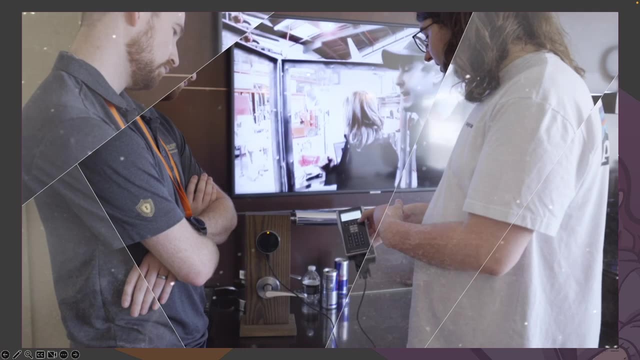 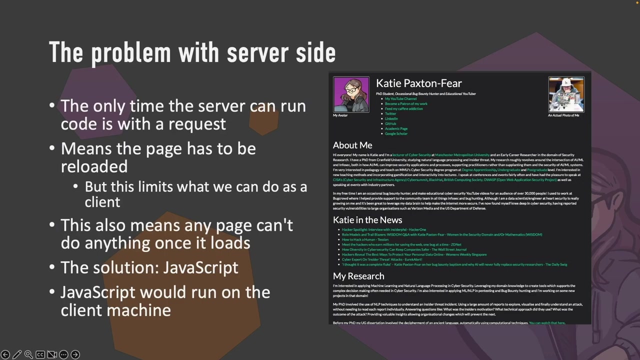 up for a waitlisted program. tell bug crowd a bit about your skills, previous certifications or experience and they'll match you up with the right program using their industry leading crowd match technology. whatever your level, there is a place for you in the crowd. so we've talked a bit about 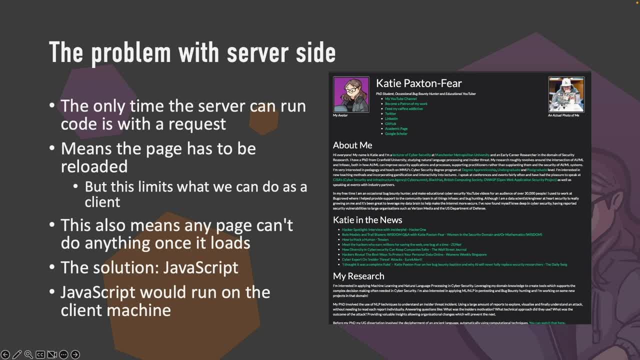 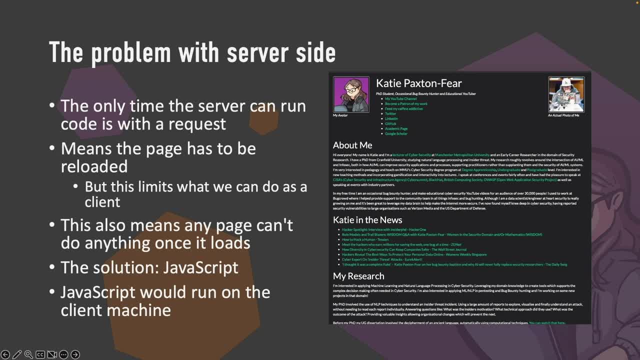 everything server side is that the only time code can run, the only time a website can do anything is when a page and when they have a request and a response. so the page has to be reloaded. but you will probably use the internet recently and you know you don't need to reload the page to. 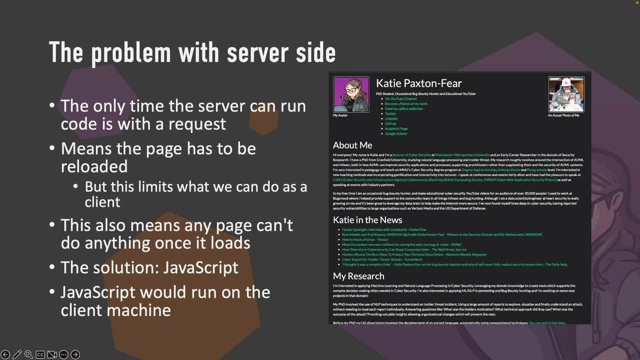 click on a button. so javascript is a client-side programming language. it's done all on your computer that renders out this client-side language, which can help do this. so essentially it allows you to run client-side code on your computer. now, because javascript is client-side, not server-side, you can actually also read javascript and you can see what, how it's being. 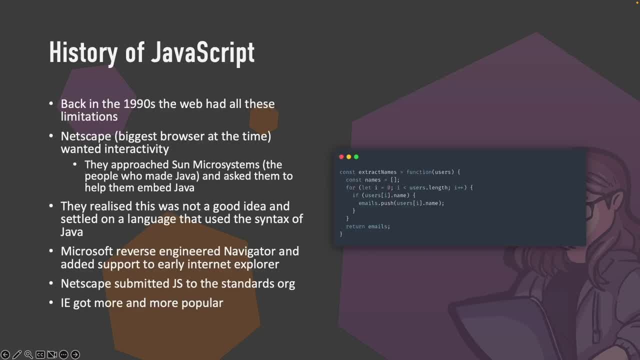 used. so in terms of the history of javascript back in the 1990s- and actually this is true for quite a lot of security issues- is the web had a lot of limitations. the modern internet is very much based off of technology in the 80s and 90s and that's actually why we see a lot of security issues. 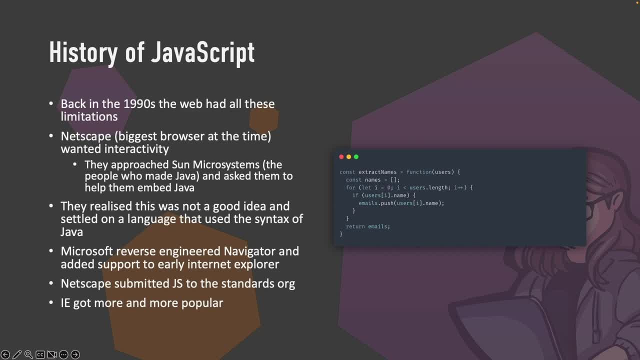 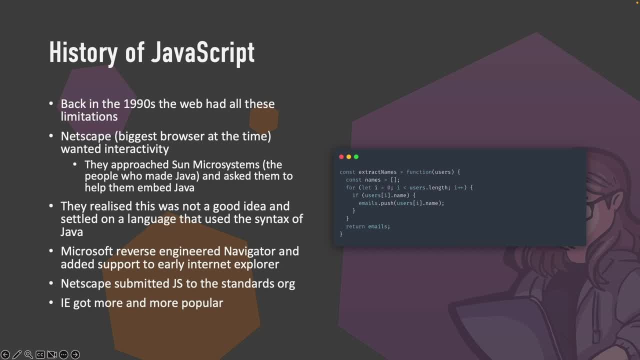 and they made java get into a website. they realised very quickly that java was a terrible idea and that's why we actually call it javascript, because it was made by the people who make java. now, when netscape made this, microsoft saw and were like we want that too, so they reverse. 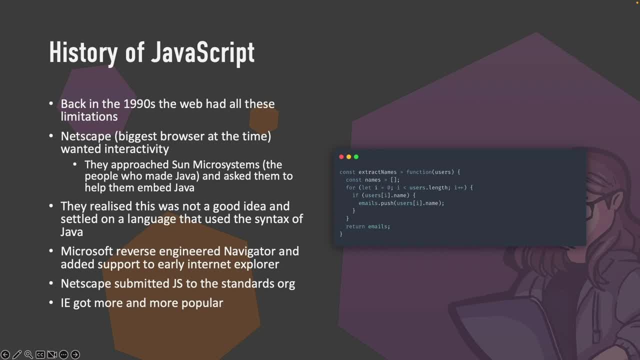 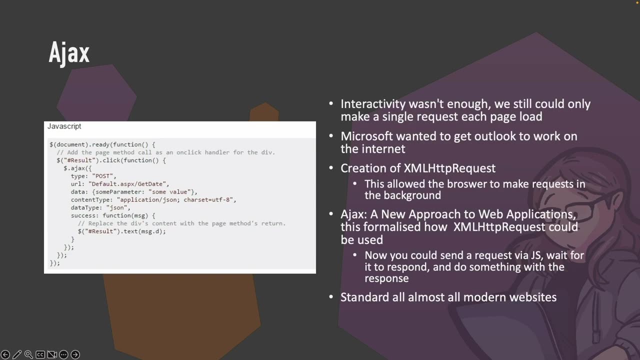 engineered netscape navigator, so that's the web browser, and added support for javascript to early internet explorer. so netscape submitted javascript to standards organisations. however, it kind of didn't really matter. internet explorer got more and more popular and with that microsoft wanted to get outlook- so that's their email client, to work on the internet. 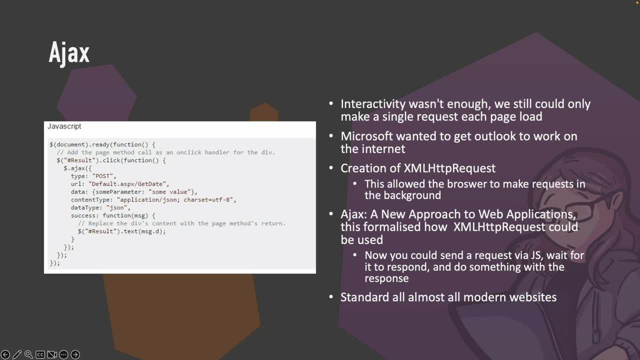 the problem is is that single activity with javascript was only so much you could still only make a single request each page load like you couldn't also send more requests, so microsoft ended up inventing xml http request. so essentially, what this technology allows you to do is make the browser make a request in the background using client side code. so now you. 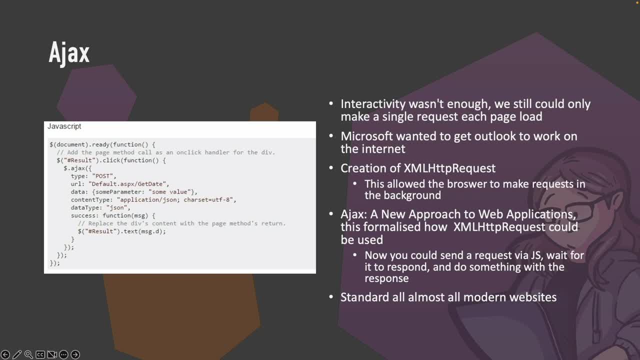 weren't limited to a single request to do stuff. you could have javascript. you know, click a button, javascript sends a request on your behalf. now you can kind of do something with that response on and make really interactive. you think about anywhere you want to do that. you can do that on your website. you can do that on your website. 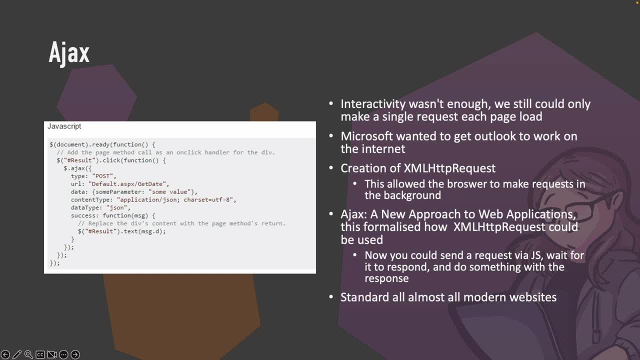 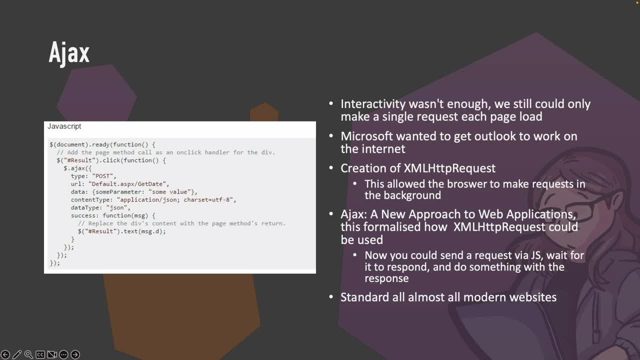 recommend hacking some kind of email provider, you will see it do. a request for suggesting more emails to put in, they'll have a request. if you attach a file, they'll have a request for actually sending an email and viewing an email. and all that is because of ajax. it's still on your single page request. 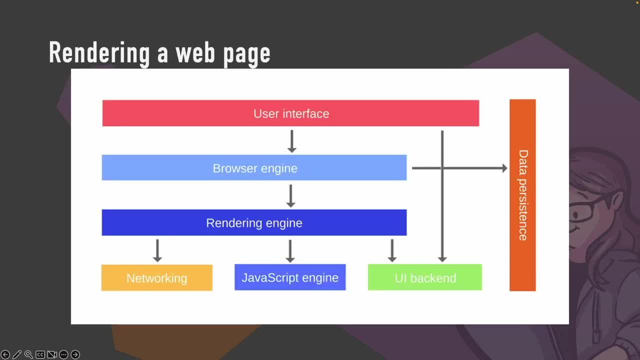 so that is the kind of standard. now this is kind of out of scope for this video, but essentially, when a web page is actually rendered, you are just getting the response right. if you go into burp and you see request response, your browser gets the response. so the actual thing that creates the 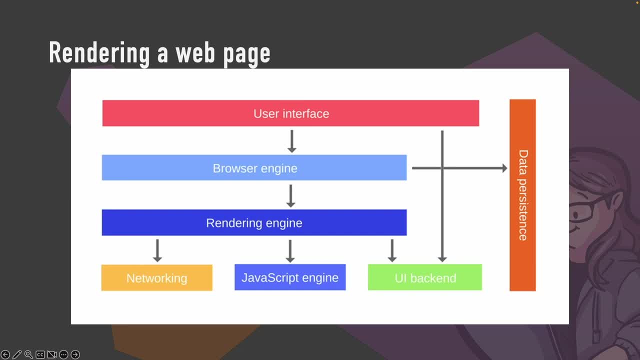 nice little pictures- is the browser engine, and for different web browsers these are different engines. that rendering engine puts stuff on the page and then, after the page is done, then we have javascript. so javascript will then run all of the code and this is actually, you know, continually running. so what cross-site script is is it's not a flaw in how your web browser reads? 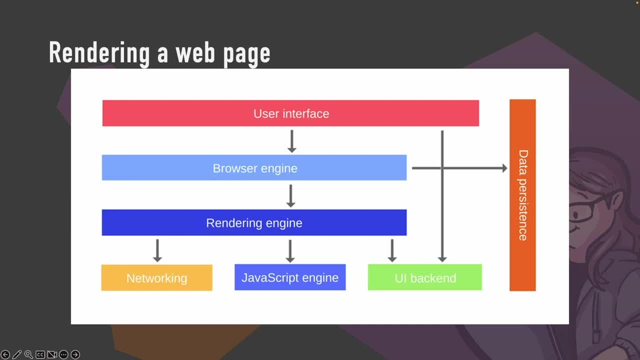 or outputs javascript. it's a flaw in essentially running untrusted code. now, javascript is kind of intended to be a flaw in how your browser reads your references. so if you have a javascript which intended to run arbitrary code like it's supposed to, but cross-site scripting kind of allows us, 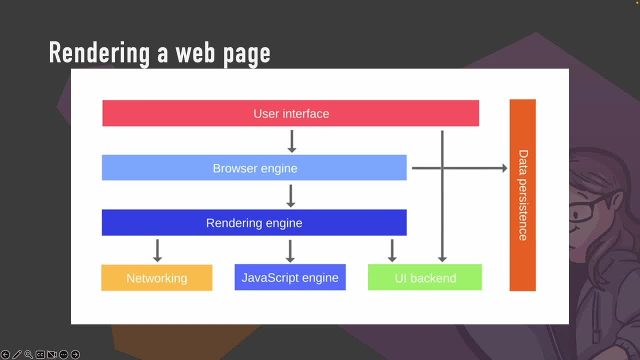 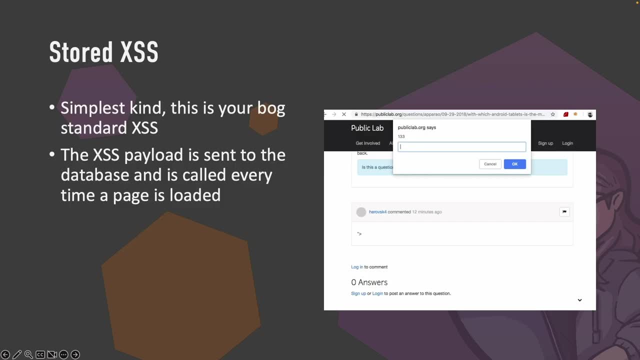 to increase the impact of running this arbitrary code, especially on behalf of, and pretending to be, a website. So there are a few different types of XSS. The simplest one is what's called a stored XSS. So a stored XSS is kind of your bog standard. 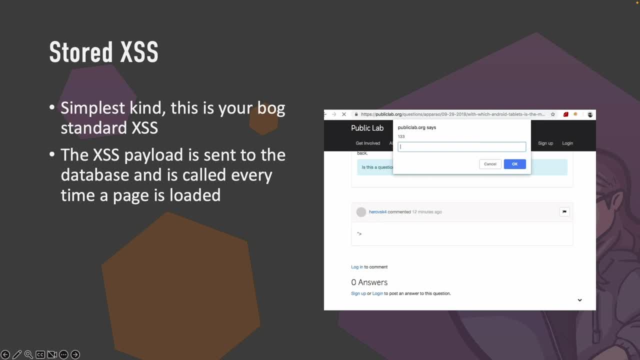 The XSS payload is sent to the database and is called every single time the page is loaded. So essentially you can put in arbitrary JavaScript. it gets saved to the database and then, whenever you load up that comment or that post or that video, the XSS payload that's in the title or the description. 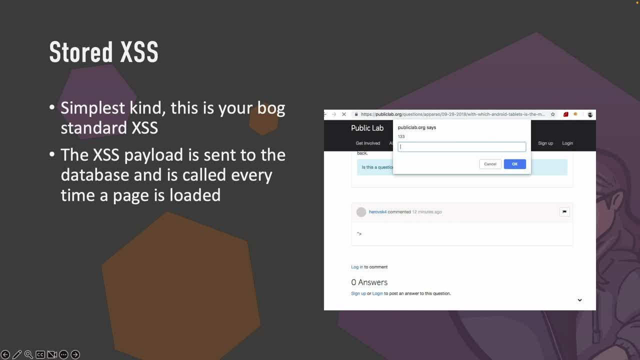 or wherever it is, will then appear on the page. This is the most impactful of the XSS types, because it's really difficult to argue that the impact is lower. The impact is obviously higher. it gets stored in the database. Now it's not necessarily a problem. 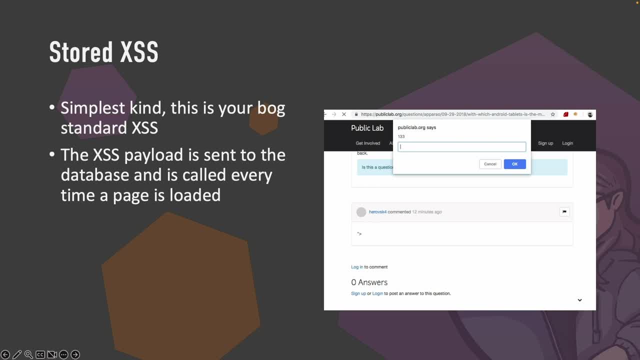 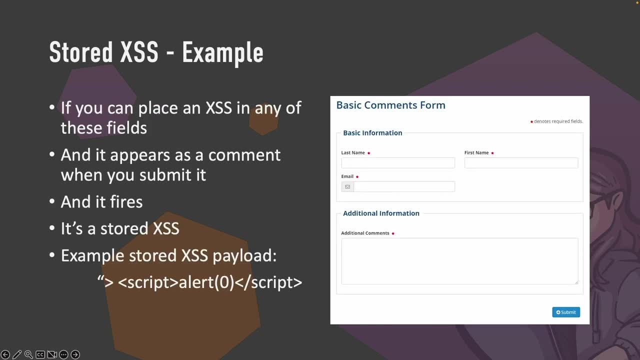 if your XSS payload gets stored in the database, The problem comes when the page is then rendering that as JavaScript, so you can see this here. So the best way to test for this is to place an XSS payload in any field on some form. 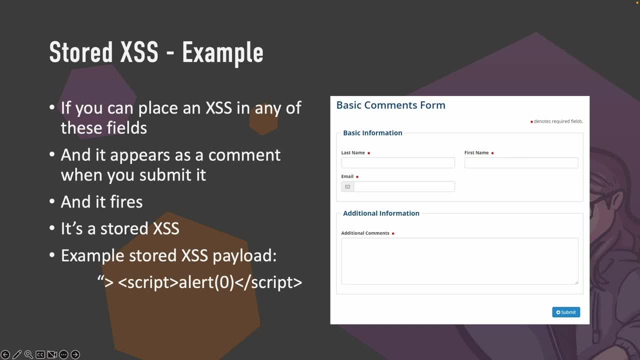 So in this case this is a comment form. So you place an XSS payload in last name, first name, email, additional comments. Then when you submit it, if you refresh the page, you can see your comments. That is a stored XSS. 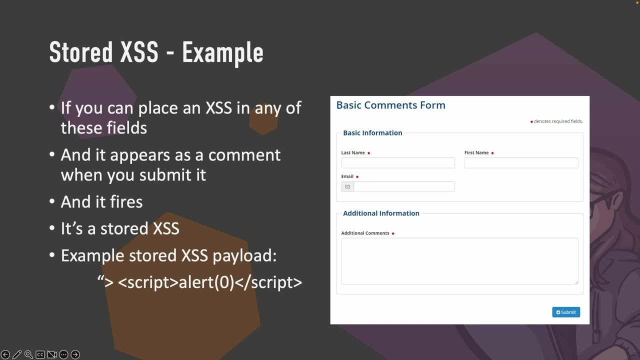 So the very simple stored XSS payload is script alert zero script. You shouldn't really stop there, though. Demonstrating more impact is how you can start to especially develop more as a hacker. You don't always need to demonstrate more impact, but if you do, you can really demonstrate things. 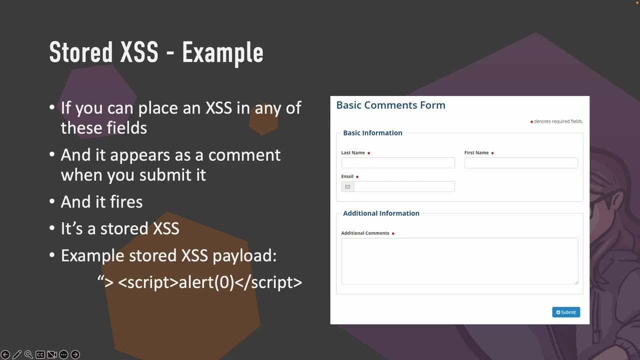 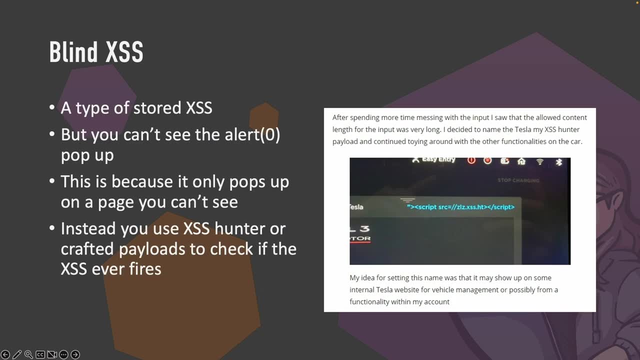 like account takeovers, right. That's how a lot of people move on From low and medium bugs into highs and crits. They're looking for that additional impact. The next option we have is blind XSS. So blind XSS is a type of stored XSS. 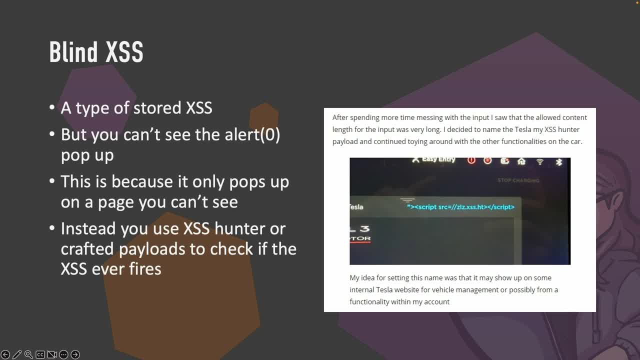 but you don't see the output of alert zero. You don't see that pop up because it pops up on a page you can't see like an admin panel. So you can use XSS hunter or crafted payloads to see if the XSS ever fires. but essentially 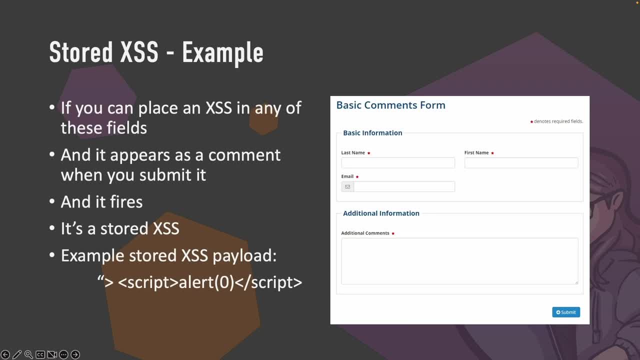 you can imagine, if we take the comment example, if a comment had to be approved by an admin, the XSS payload may appear on the admin control panel right. It's also really common in reporting posts in reviews in. you know, you got to think. 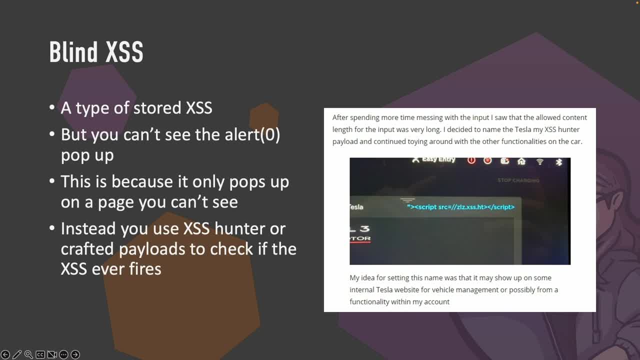 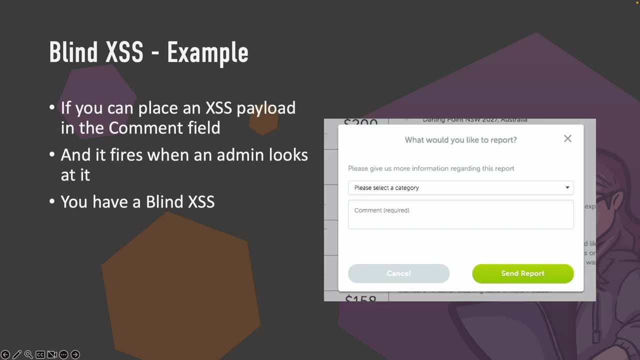 where does this go into a administrator control panel? Where would that go? What would it look like? And then we have another example of here of a report field. So you're looking for places where an admin would look at it but you wouldn't necessarily be able to see. 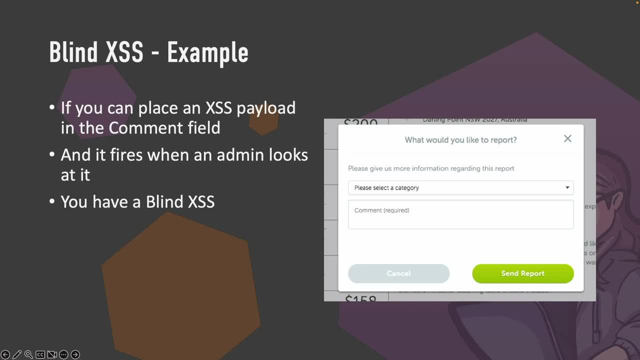 that is a blind XSS. It is still fundamentally a stored XSS, Like at the end of the day it is just a stored XSS. It's just a different type And these require time. but I, in my experience, I've seen that XSS- blind XSS- tends to be. 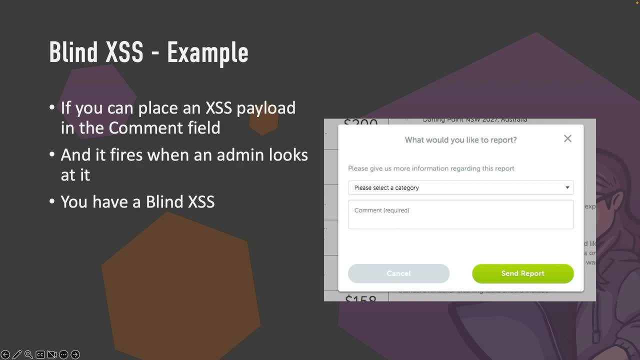 one of the most common types of success that gets picked up. It's paid out quite a lot because it tends to be what developers haven't fixed yet. They don't really consider the impact of it. So if you are hunting for blind XSS, you've got two options. 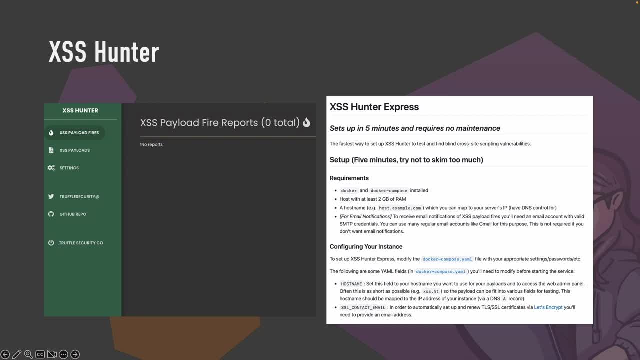 So there's a piece of software called XSS Hunter. It was shut down a few months ago, but there's now XSS Hunter Express, which is like a self-hosted version. You can see the instructions are really really clear, super easy. 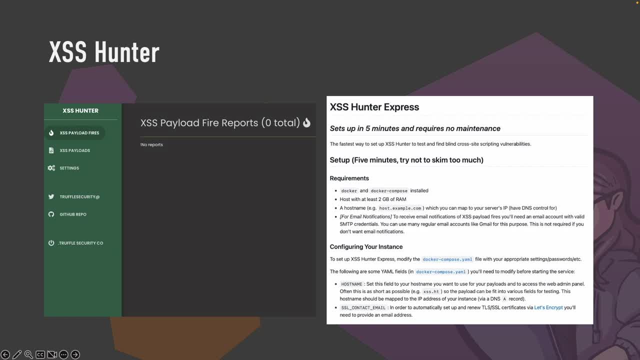 You can get set up really, really fast, Really quickly. Or you can use Truffle Security's XSS Hunter, which claims to be a kind of more privacy focused XSS Hunter, Though there was some controversy with them storing data, So if you are worried about that, 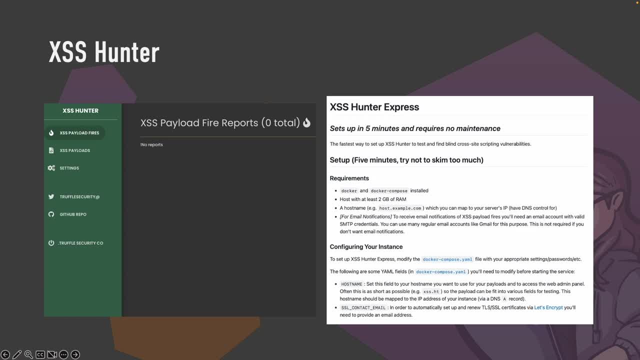 just do XSS Hunter Express. Now the one downside is for a lot of blind cross-site scripting. you need really short domain names, So these can get very expensive very quickly. So it's worth having a look and seeing whether or not this ends up being worth it for you. 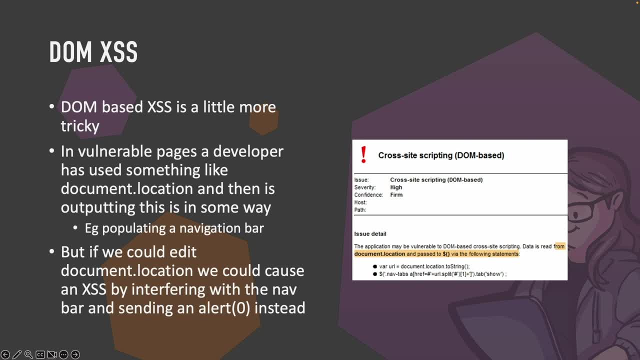 Now the next type of XSS, and the one that I found is a DOM based XSS, So they're a little bit more tricky. So in a page vulnerable, two Dom based XSS, something is happening that's using the DOM of the page. 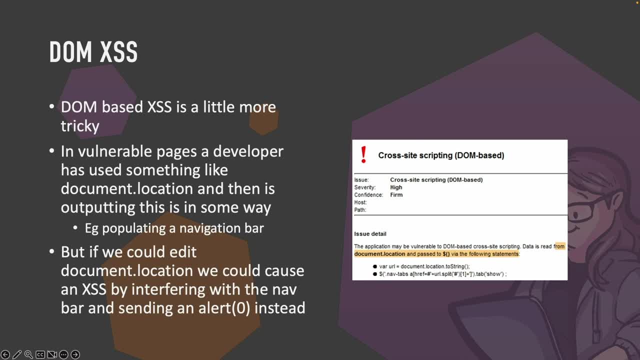 So for example, maybe it's using something like document, document location, directory, Registry, table, ال؆ �. populate the navigation bar and add where you know whether or not that's the selected link so as long as you can edit document location you can interfere with the nav bar but really this accounts for any 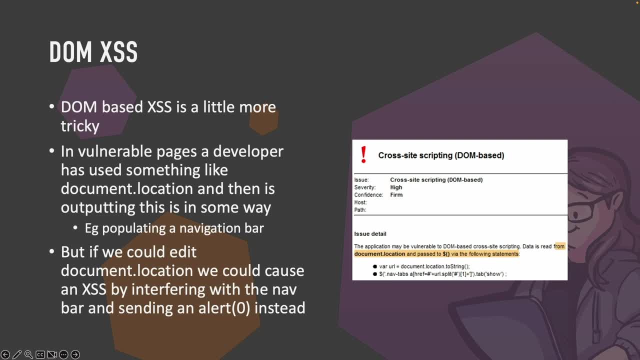 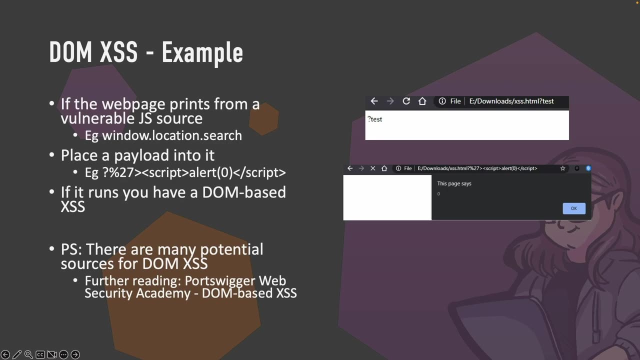 page which is using javascript to do something on the page. maybe that's populating a navigation bar, maybe that's populating a form with existing data that you sent before. that was the bug that i found. that would be a DOM based xss, so if the web page prints from a vulnerable javascript source, so it 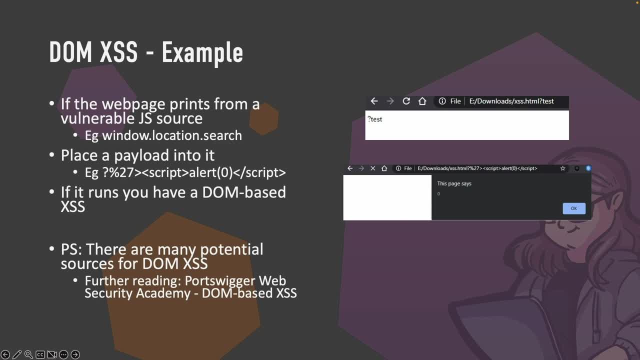 needs to have some kind of javascript that's editing the page after it's loaded. so maybe that's getting the window location search, maybe that's grabbing the parameters. this takes reading the code. you, you. it's well worth it, though. i promise it's well worth learning javascript. 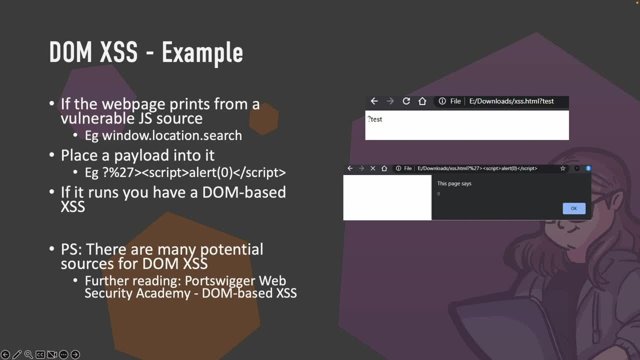 there's a book called javascript for hackers that, if you're familiar with javascript, well worth reading. if you're not, i'd probably give it a skip or do a tutorial first and then read the book once you kind of get your confidence really worth doing it by. so then you 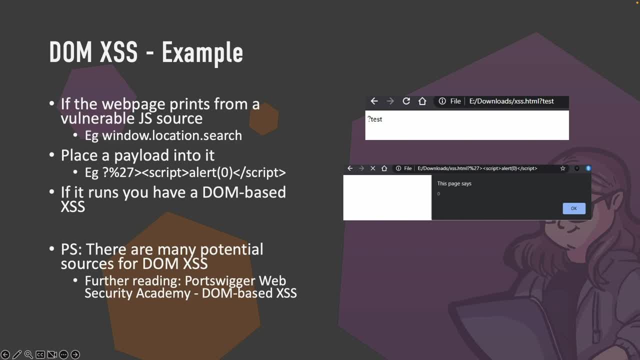 place your payload into that vulnerable location. so you can see on this example here that it's grabbing the parameters. so we just have to set and you see it's printing out the parameters. we just need to set the parameter to be script alert zero. there are so many potential sources for DOM based. 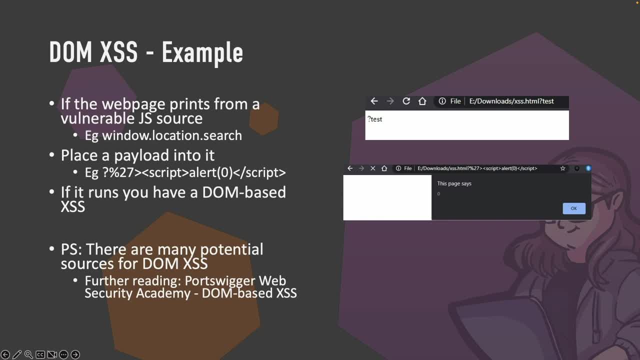 xss. so if you're familiar with javascript, you're probably familiar with javascript, but if you're familiar with xss, it is such a broad vulnerability category. i really recommend port swigger web security academy just in general, because i think it's really great if you like to learn in more of. 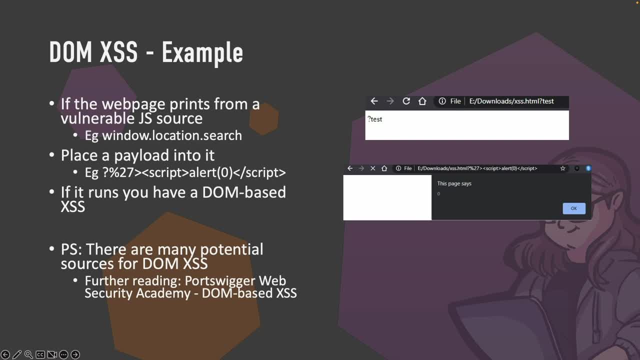 a classroom environment that gives you kind of like structured labs and then it builds on them and you can look at their information pages plus, as you do it, you're actually getting like your burp certification. you still need to pay for the exam, but you're doing all the labs that you would. 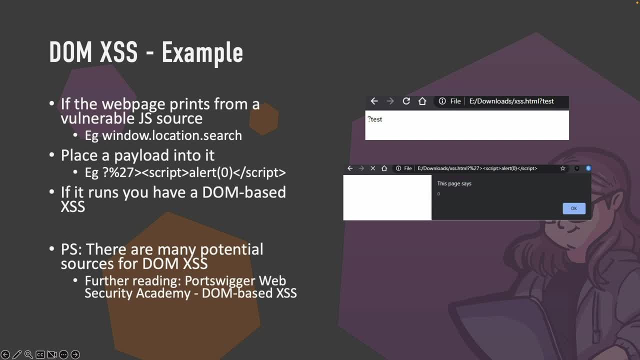 have to do anyway. so i really really recommend javascript for hackers. so if you're familiar with javascript, you're probably familiar with port swigger web security academy. it's all free, there's tons of videos and actually there's loads of videos by the community as well, so it's not just 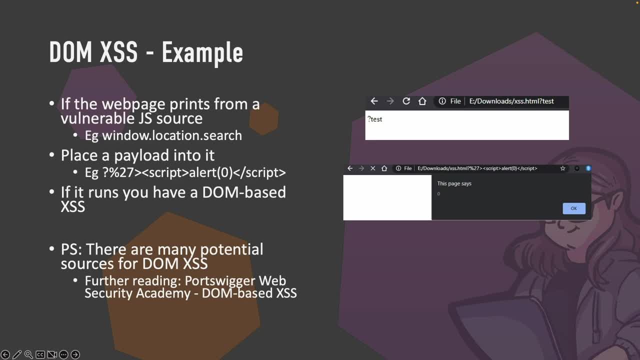 there's a bunch of people who think it's worth doing, but i really recommend it because i there's so many different ways to cause DOM xss. i would say, if i, if you were like katie, what kind of cross-site scripting should i look for? i would say: learn to read javascript and DOM xss. and i'd say: 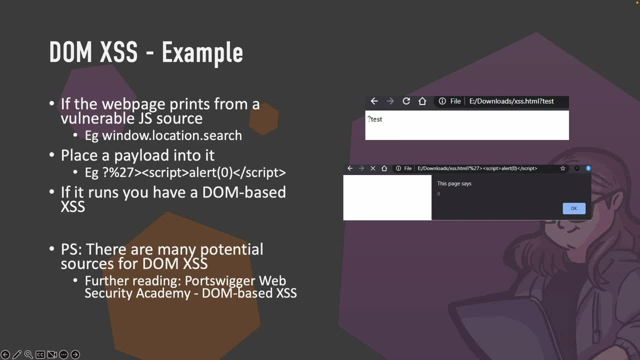 blind, xss, especially if it's a newer bug bounty program or it's something that hasn't had a lot of eyes on it yet. x, blind, xss is a bit more common then. but being able to read code, being able to read javascript, it's such a major advantage. 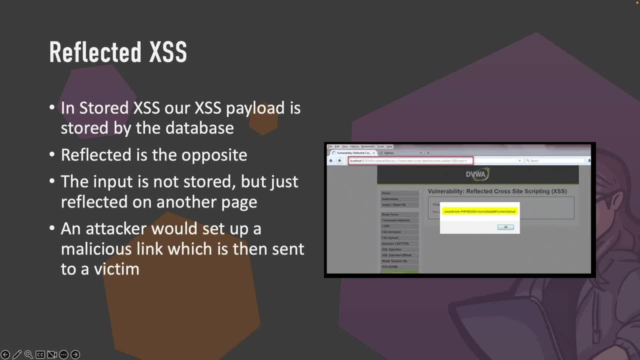 so the final type of actual valid xss is what's called a reflected xss. so we've got to compare this to the other ones we looked at. so in stored xss our xss payload is stored by the database. it will appear every single time it's stored in the database. it will appear every single time. it's. 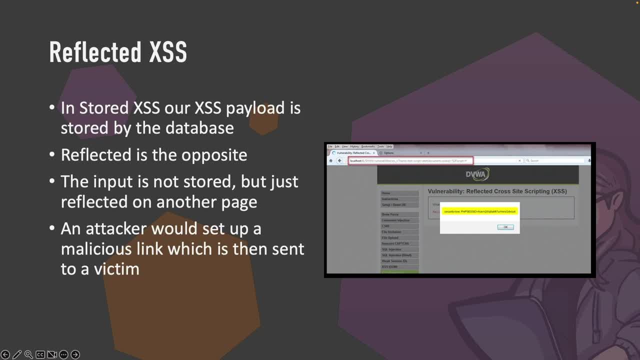 that that comment or that post is loaded up, reflected, is the complete opposite of that. the input isn't stored, it's just reflected onto the page or on another page. so you can imagine a search bar where it's: you know, google. if you type in a google search, it will say search results. 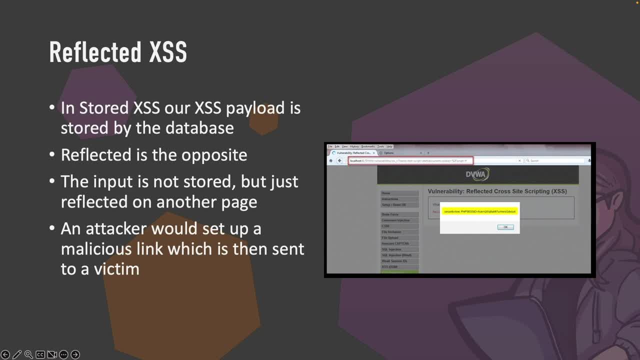 for whatever you searched. that is then where you'd have reflected cross-site scripting, so an attacker would essentially have to send this full malicious link to a victim, and the victim then need to click on it. this is why reflected xss has a much lower severity in a lot of situations. 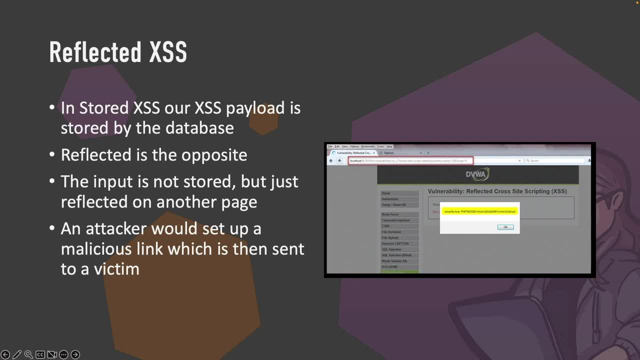 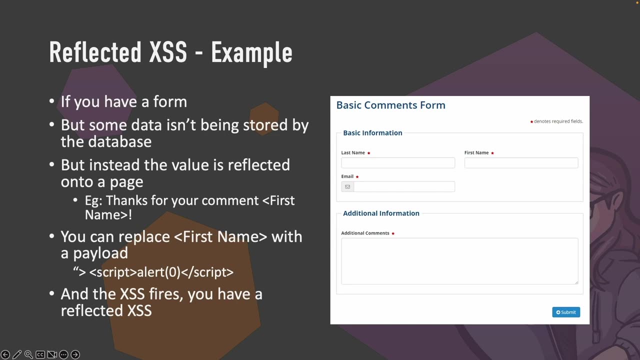 because it does take social engineering to actually get someone to click on it. it's much better if you can convince or you can store something in the database, right, you don't have to convince somebody. so let's have a look at example so we might have this form. maybe it is. 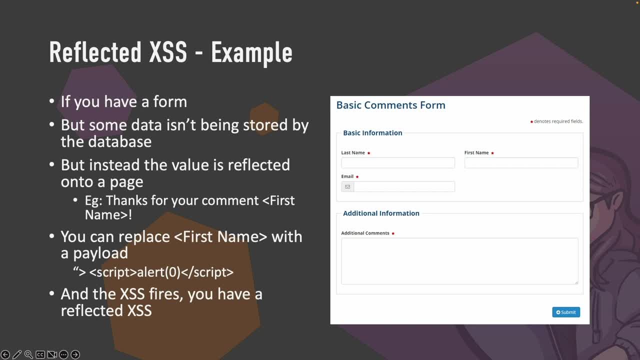 being stored by the database. maybe it isn't, but the next page that we're going to be looking at is the one that says thank you for your comment, katie. thank you for your comment, whoever right. so if that first name is then reflected onto the page, you can edit that first name to be an xss payload. 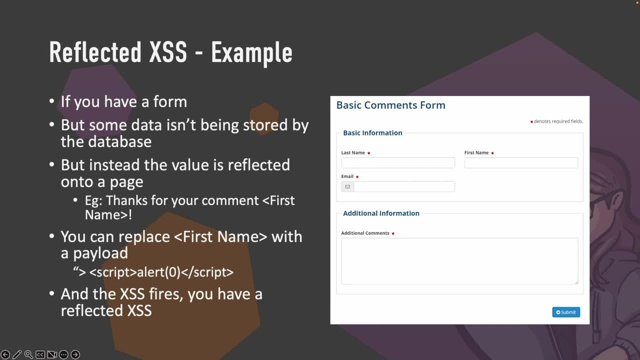 and if you can refresh the page and then cause that to appear with your alert one, that is a reflected xss, and this is why i think it's kind of important to learn the further impact of scripting, particularly things like account takeovers. things like xss hunter make this really easy, because they will grab things like cookies. 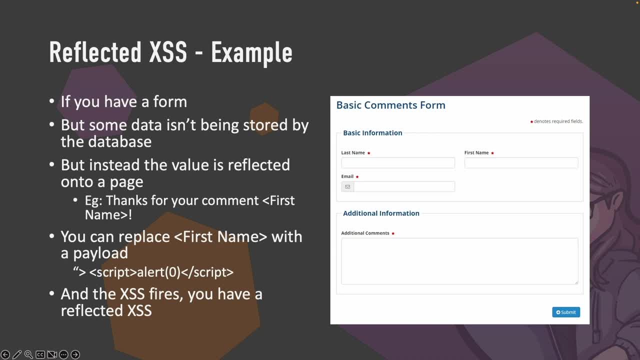 from the page that you might be able to reuse if the session is still active. but for quite a lot of them, you're going to be looking at csrf, which is another type of vulnerability that you would have to chain together again, especially if you've got a reflected xss. a lot of people will say, okay, yeah, 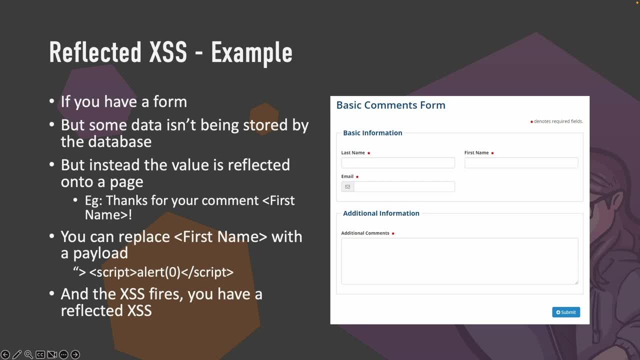 but what's the impact? well, the impact is you could steal somebody's cookies, but we don't have cookies in http, only you can go. okay, you might be able to cause an account takeover. okay, how? again, if you can demonstrate that further impact. that's what bug bounty programs want to see. the final type of xss is what's often called 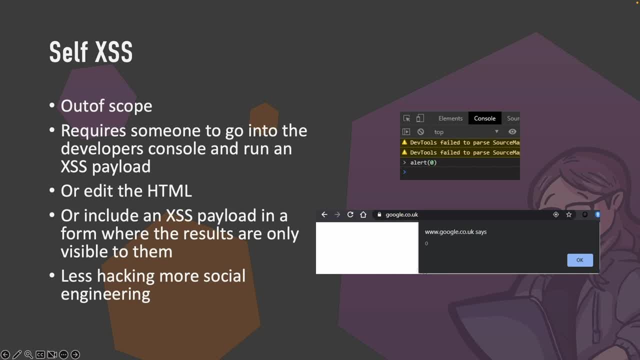 self xss and this is usually considered out of scope or na. this usually requires a high amount of social engineering, so it requires you to get them to open the console or edit html or include an xss payload in a form where the results are only visible to them. to be able to get somebody to do that is going to be. 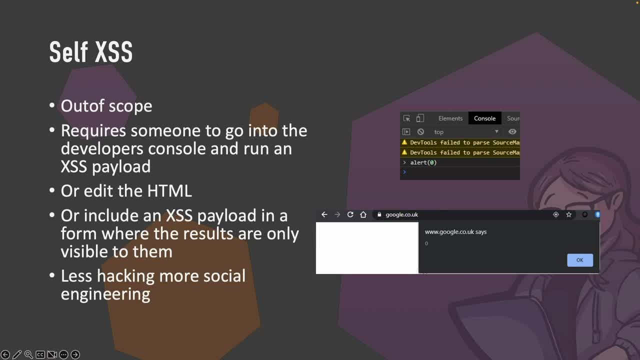 tricky like. it's not even just an email where you can send a malicious link. it's that one step further of saying, okay, do step one, then step two, then step three and then step four. and, honestly, if you're going to do that, you're going to have to do a lot of work and a lot of work and a lot of. 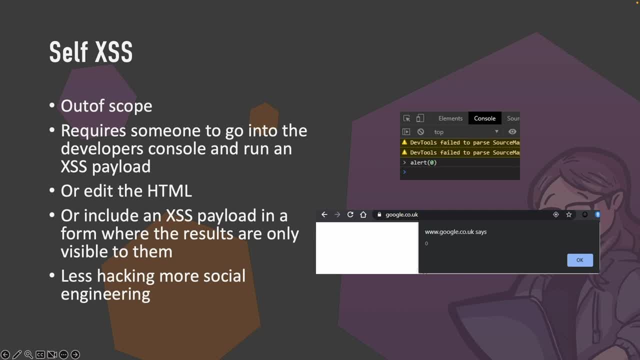 effort and they're still following you. you may as well just ask for their password, because they're probably going to give it to you, right, self xss is just that other level of okay. this is yeah. this is going to be really hard to get somebody to do, so. it's less hacking, more social engineering. 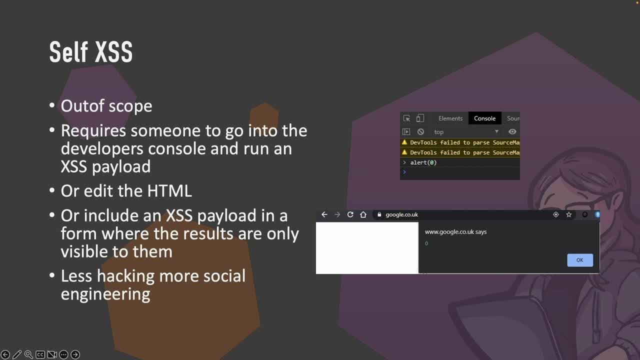 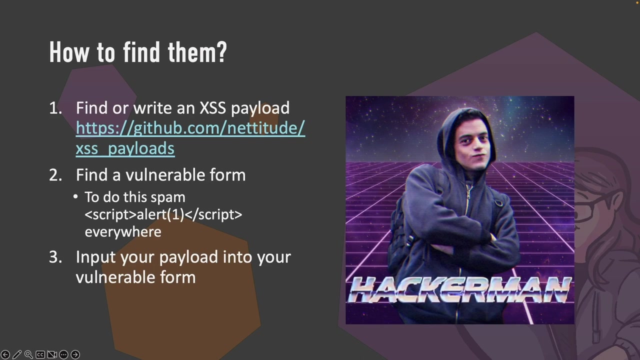 in some cases, if a program does allow social engineering, this might be considered in scope. but i will say very few programs allow social engineering and even then it's probably not a huge like amazing finding anyway. so how do you find xss payloads? you can find or write an xss payload. there are a bunch of them online. i will say that. 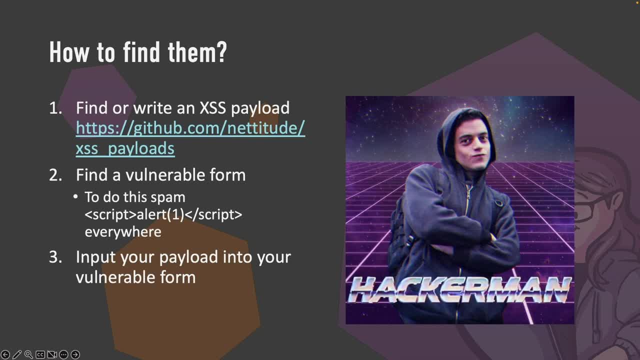 just copying a big list is not the best way to find cross-site scripting, though i cannot argue with the fact that people have got results this way, and maybe i'm just bad at it. i will freely admit maybe i'm just bad at it, but i will say that it's not the best way to find cross-site scripting. 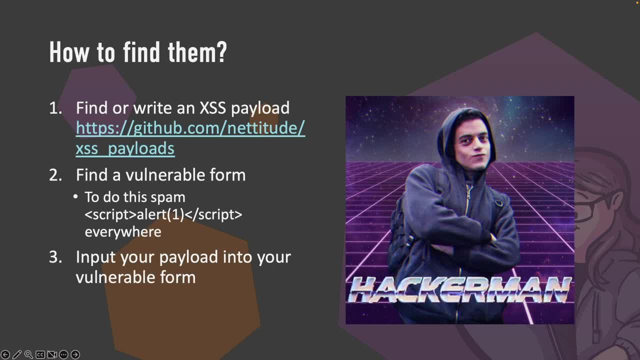 maybe cross-site scripting just isn't my bug and i just don't get it. so you want to find or write an xss payload? now, the reason why i say find or write is because often, based on context, you need to know how to make changes to that. a lot of the WAF bypasses that you see are because there's a 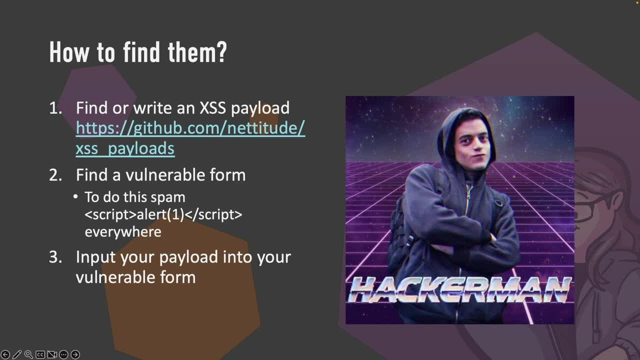 lot of the xss bypasses are because certain characters are being filtered out or because in certain context some things may be like passing differently or being saved differently. i'm going to put this in the comments, but there is a really great infographic made by some dev where he breaks down what an xss payload looks. 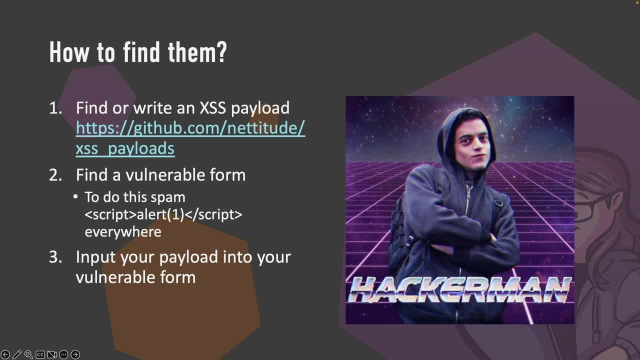 and why it's there learning that. why is so so important? and that goes for, i think, all bugs. simply spamming script alert: one may work right, it may work eventually. but if you can understand how to write an xss payload, why something works, why a specific payload is is working, you can get much better results. and 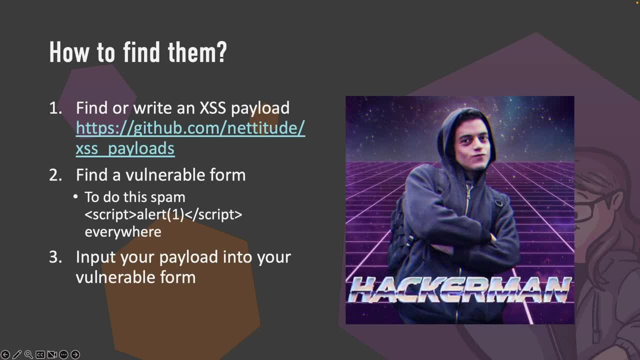 more impactful results. saying that, i will say: a lot of the testing, at least initially, for cross-site scripting is often script alert one. now, depending on how that payload is then passed by, the vulnerable form kind of determines your next play. so is something being filtered? is the script alert? 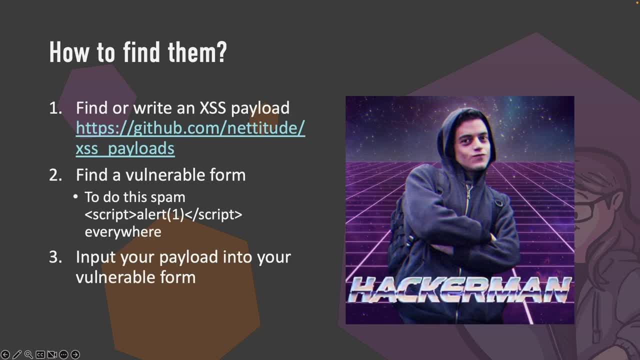 one just appearing in the script alert one. is it being filtered? is it being filtered? is it being on the page? is the script appearing but not the alert? is there, i don't know, a filter on the little angled brackets? all of those will determine kind of how you approach it next time. so maybe you have. 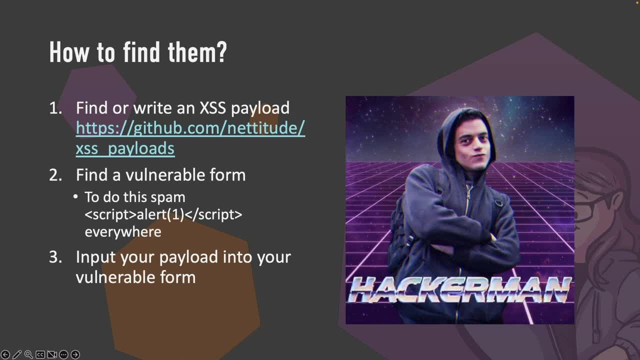 to not use script tags. maybe you have to use a javascript url slug instead. maybe you can't use alert one. you have to use input. maybe you have to use a url right, you have to load a script from a source. all of that is going to be dependent on the type of form. 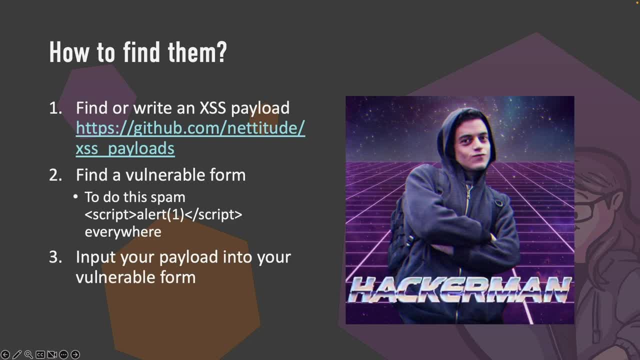 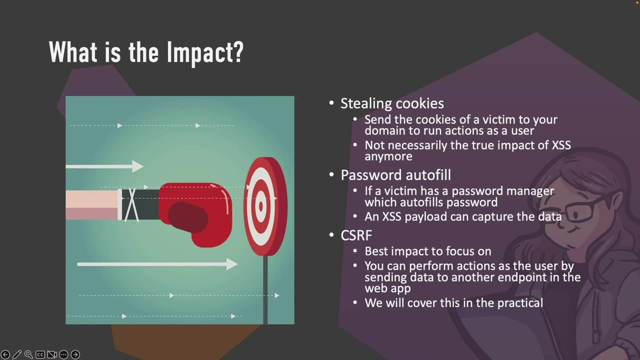 you're looking at and when we go and do the live demo in a few weeks- and i'm going to talk about actually bug hunting- we're going to see this in practice and see how you would go through these steps. so what is the impact of cross-site scripting? there's kind of three key impacts. first, 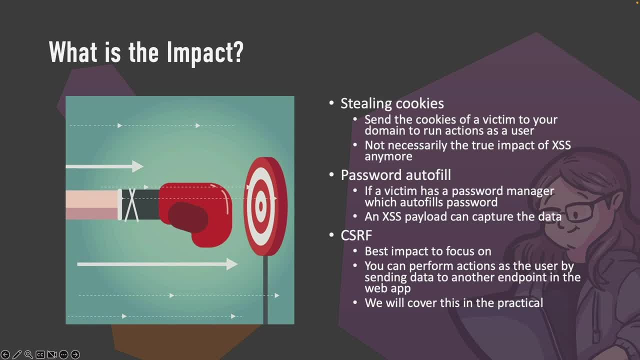 is stealing cookies, so it's not necessarily the true impact of it, but it's the impact of the access anymore, because very few cookies are http only and kind of won't necessarily work. the other one is password autofill, so if a victim has a password manager which autofills a password, 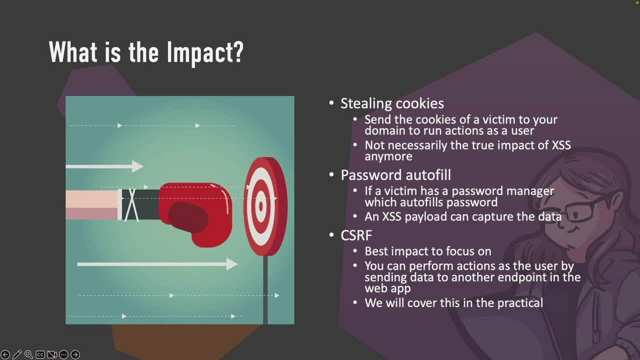 an xss payload can actually capture that data as like the password manager is typing it in. however, the big impact is what's called csrf, so that's client-side request forgery. that's something we'll be seeing kind of later in the day, so that's a big impact. and then the other one is the impact of 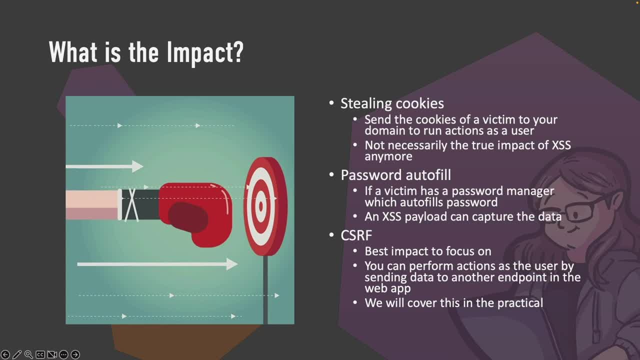 cross-site scripting. so that's kind of later on when we start to look at other types of vulnerabilities. but it's essentially this idea that you can perform actions as the user by sending the correct data to another endpoint in the web app. so you can imagine your xss payload. 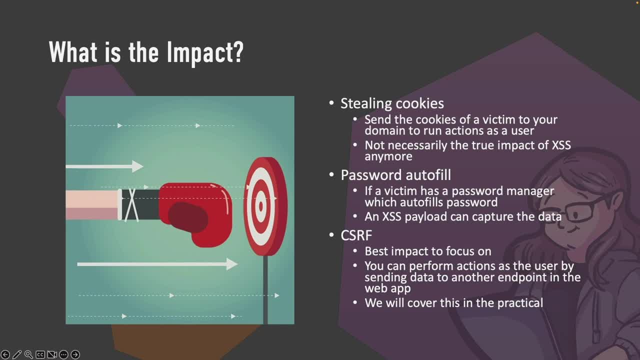 wouldn't say alert one. it would instead say: hey, can you change this password for this account to just be the word password? we're going to cover that again in the practical live demonstration when i do this all the time. so that's a big impact. and then the other one is the impact of 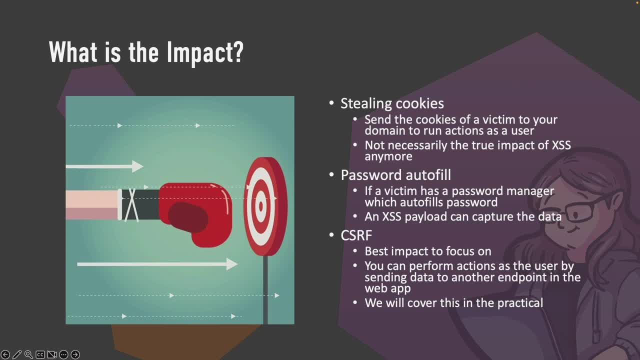 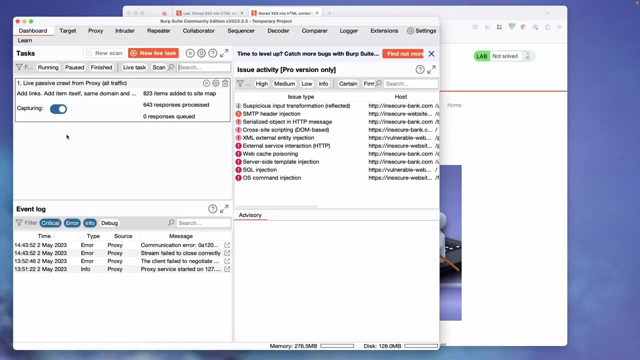 virtual life for you. so let's have a quick look about cross-site scripting in action and specifically when we know something's not vulnerable. so give me a moment and i will get set up here, okay? so we are back and, as you can see, i've got a web security academy one up. i've got 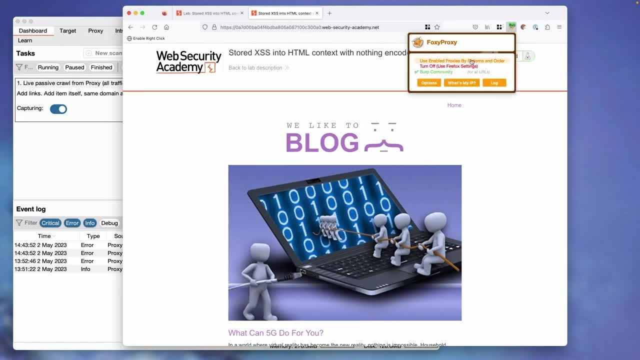 burp running in the background and i'm using foxy proxy to actually connect to burp. if you're not sure how to get burp set up, you can see my earlier video on how to get burp set up and i'm going to show you how to actually get a hacking setup together. but the first thing you do whenever 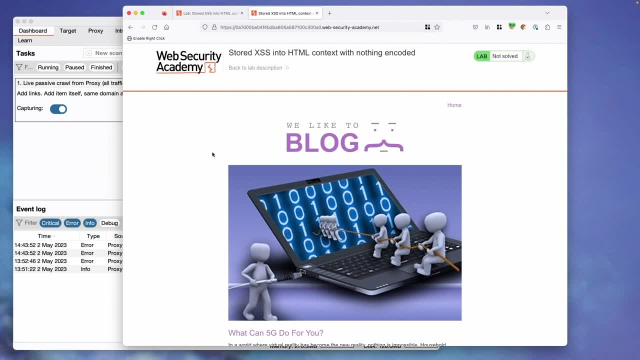 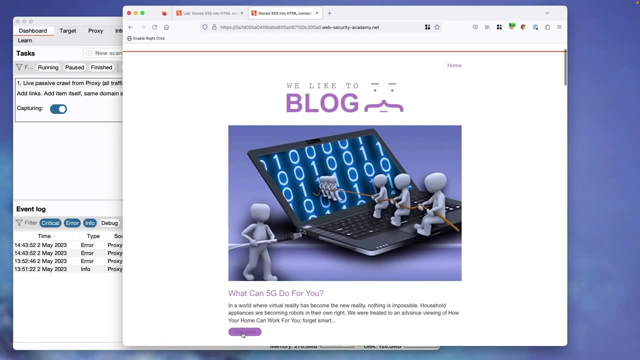 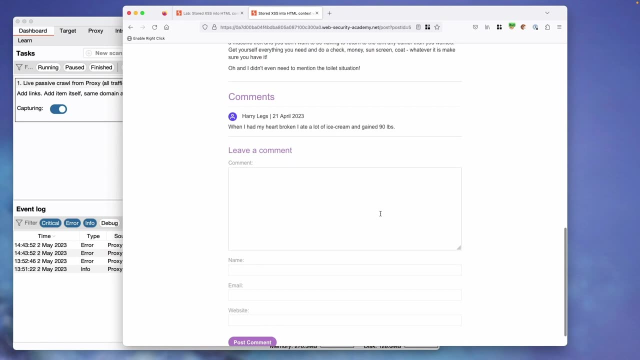 you're approaching any target doesn't matter if it's a ctf, if it's a regular website. you always look at what you can do as a user and try and understand how, what you're supposed to, how it's supposed to work. so you can see it's a blog, we have posts, we can view a post and we can have. 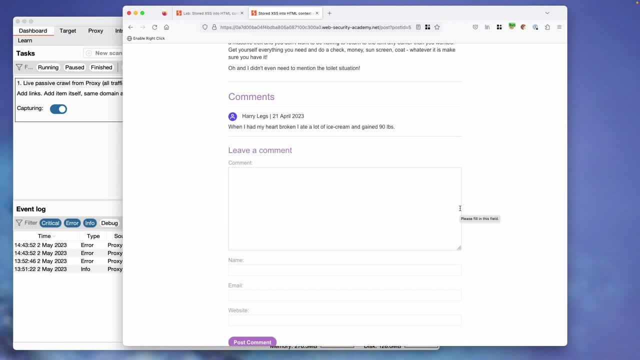 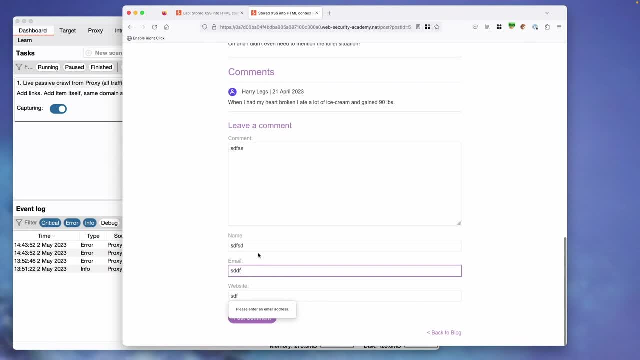 what the requirements for a comment, for example, and we can see here: okay, it needs an email and if we try and post a comment, and in this case it needs to match the requested format, so this probably does need to be a url. i'm going to press post comment and i'm going to go back to 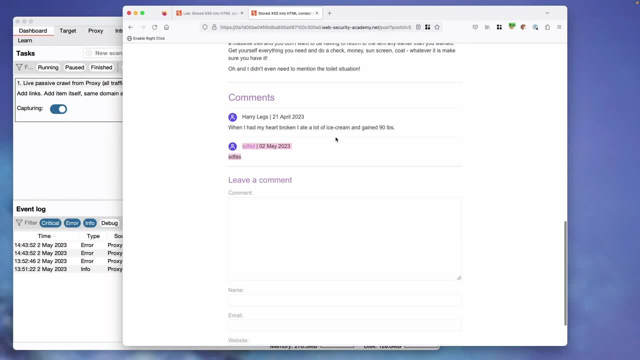 the blog and scroll down, i can see: okay, i, i've got a comment that now appears. that means that this is a stored. it's being stored in the database. right, it's. there's nothing in the url. that's changed. it's all. if i just click again, it's all. 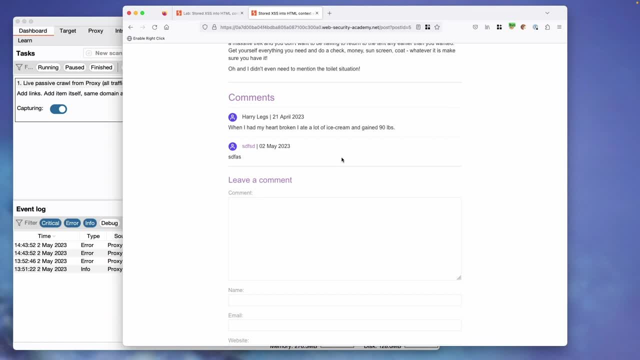 just loading up from the database. great, so we know it's going to be a stored something. now this is where we start to think about xss. so there's lots of different right ways to write xss based on the context in which it's in, and i'll show you how we see that. so i'm going to go here and right click. 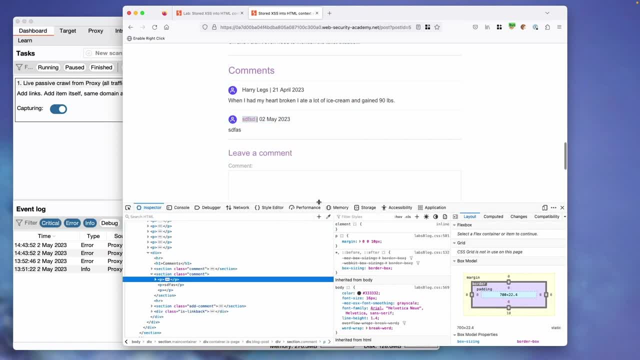 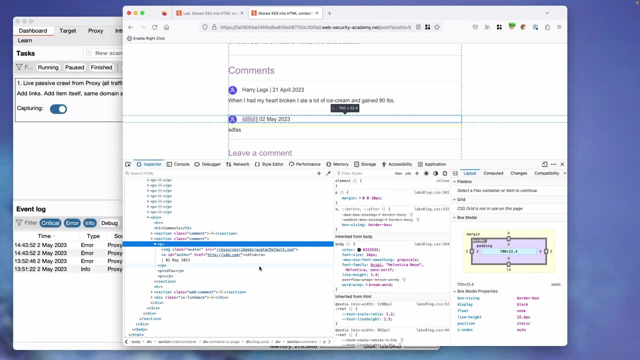 and i'm going to inspect the element yeah and see where my comment is appearing. how is my comment appearing and how is the values that i typed in then being put together to make this website? so here we can see that the url has ended up in an href, the name has ended up over here and the value has ended up in a paragraph tag. 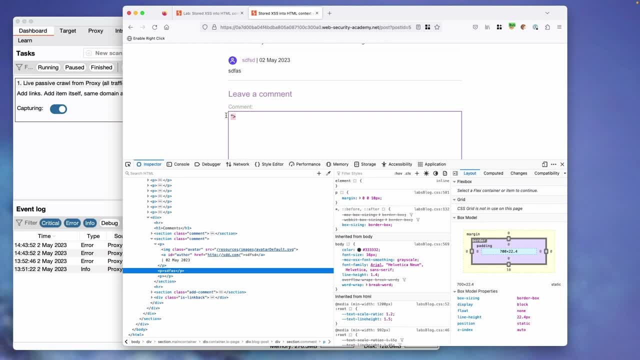 so often you'll see success, payload start this. and that's because it's saying, hey, can you close the preview? well, such a listen to what my comment is. so you guys can't sell you what that's saying previous tag. but we don't need to in this case because none of these inputs, apart from the href, 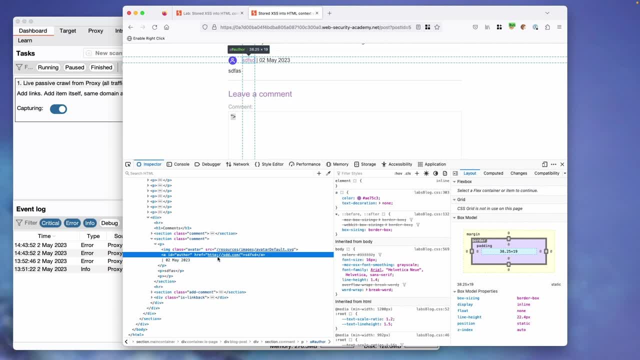 need closing right. so if we look at this, we can see if we were to just inject here, for example, we would have http slash, whatever, then we'd close it, then we'd input our xss. but if we're trying to inject into the actual comment here, we don't need to. so we don't need that because we're working. 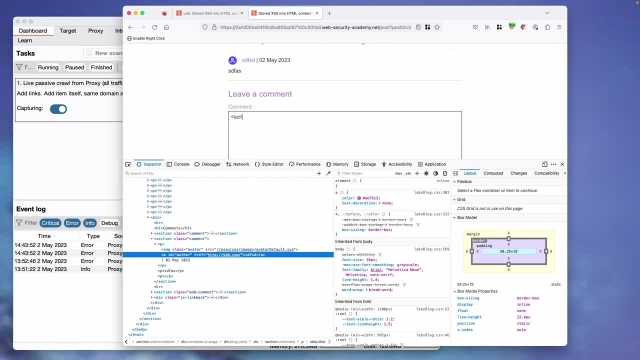 just in html, we can start by doing a script, script alert one, and then close the script tag, like so. so it's going to be the same for the author. here again, this is our name, but it's not being stored in something, so we can just copy that for the name. we know that the email has to. 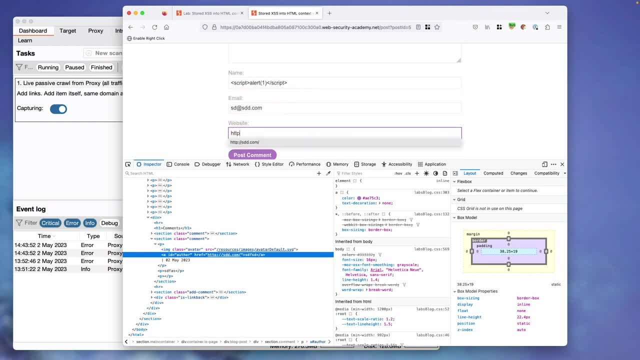 follow the format of an email and we know that the website has to follow the format of a website. so again, we're going to do a script alert one and then close the script tag like: so, okay, the two injectable fields, we know must be the comment and we know must be the name. 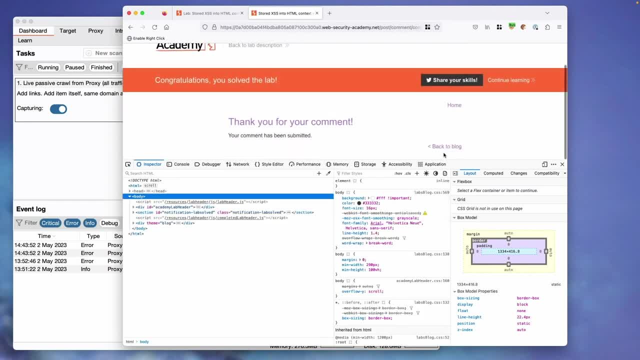 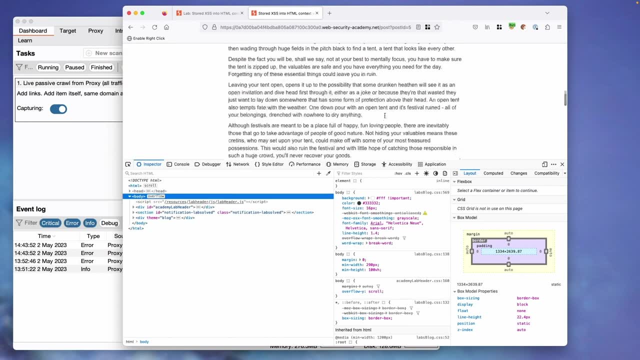 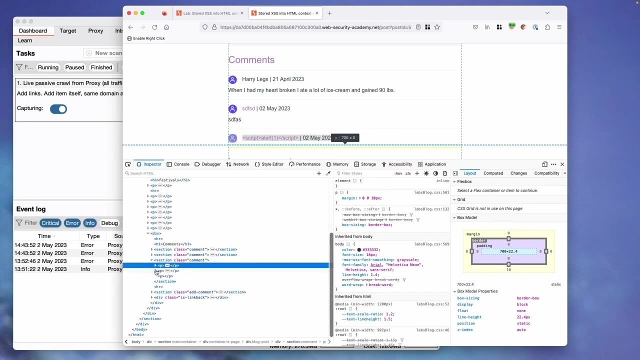 so we're going to press post comment and then we're going to go back to blog and you can see the xss payload has appeared. but why has it appeared? well, again, we're going to get up our inspect element here and take a look so we can see that the xss has fired in this paragraph tag. 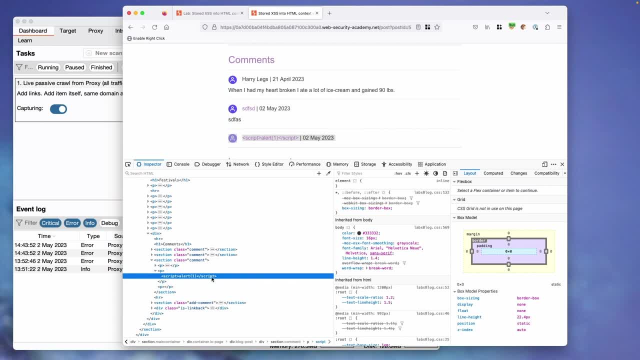 because we can't see anything, because you can see here, you see how the xss is fired in and we can see that the xss is fired in and we can see that the xss is fired in and we can see that the xss is fired in and I see that the xss is fired in and we can see. 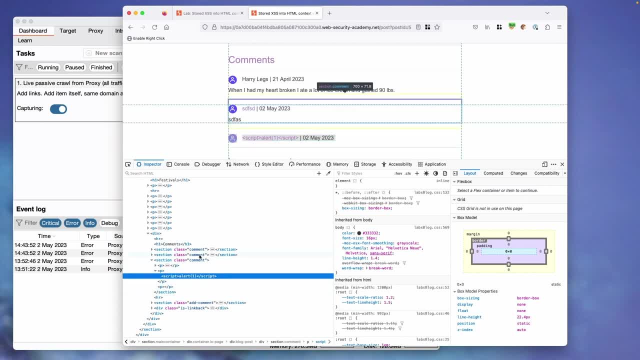 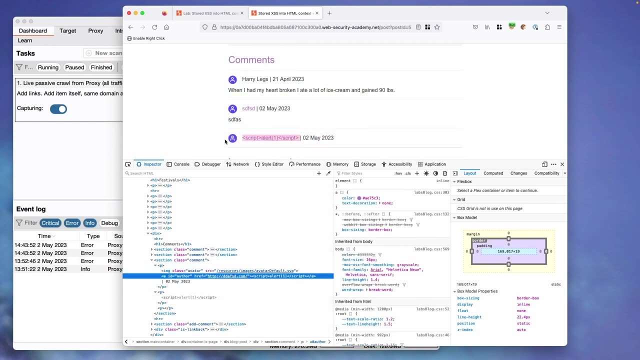 how this has gone. gray in in here. this is being read as javascript. that's saying, hey, this is javascript code. I want you to run this. that's why we can't see anything. but importantly, it does appear here. we can see script alert, one script now. whenever you see that, that's when you know. 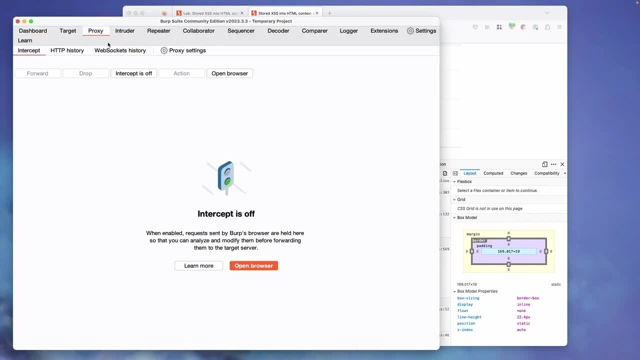 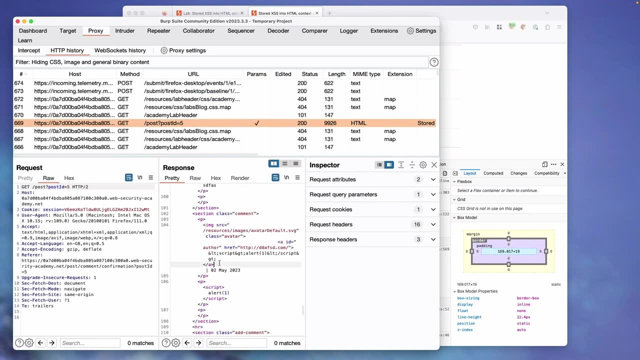 something is not injectable because if we actually have a look at our http history here, this one- and we scroll down here- is the actual result of this. now, this is automatically encoding using html encoding. so while it's not the literal character of like a less than or greater than, it's this at lt, lt for. 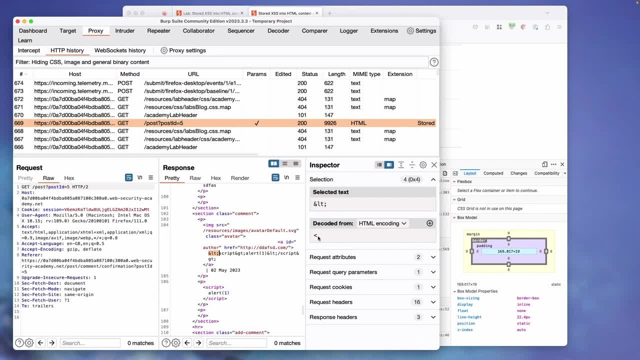 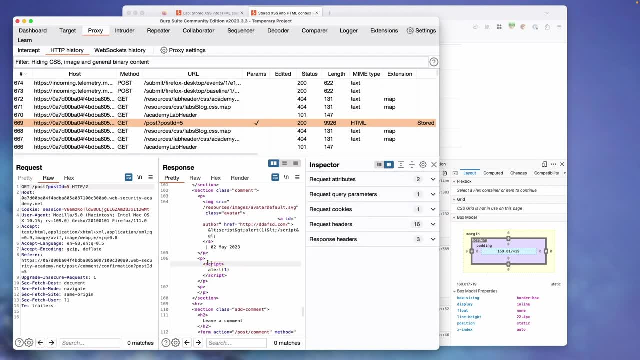 less than symbol, so that turns into that symbol in html encoding, but it's not being read down here as html itself. so whenever you see this, this is not injectable in in the same way. so this is where you have to start being creative, and this is actually where the difficulty of cross-site. 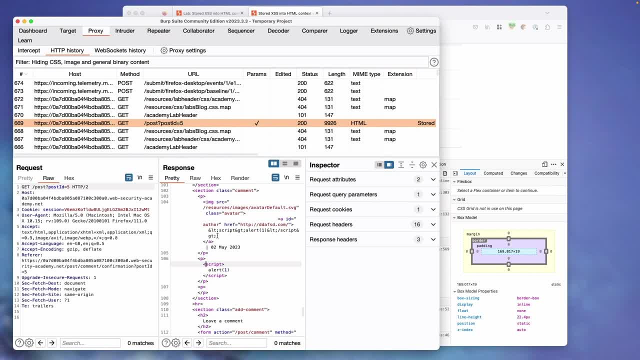 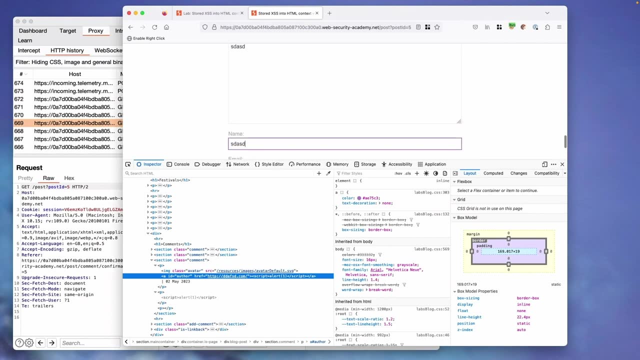 scripting really kind of comes in because you've got to figure out: okay, i can't do a less than or a greater than. it just won't work. what can i do instead? what other payloads can i try? so you might say, okay, maybe i can mess with the url, maybe you go in here and you try and put in something. 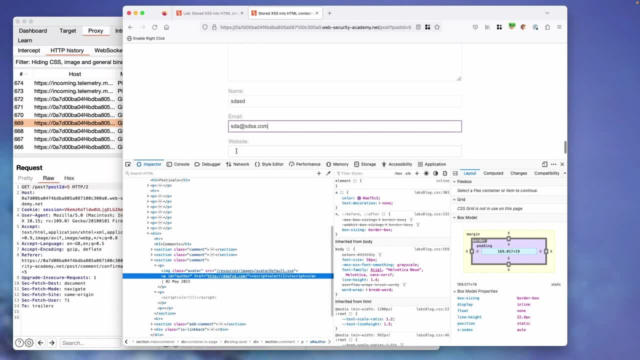 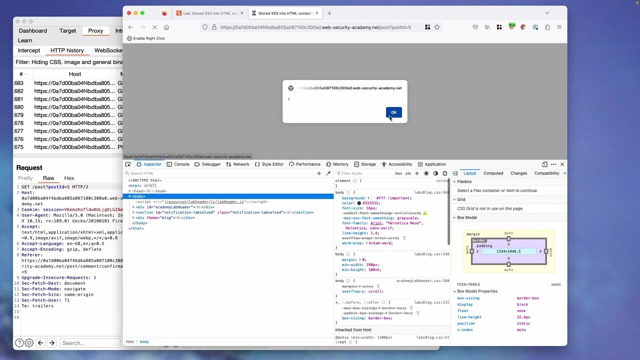 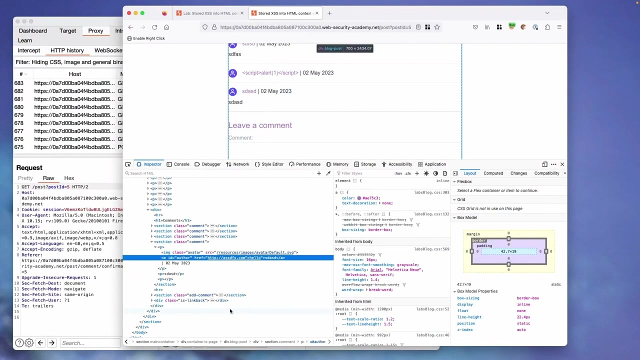 something whatever as an email and maybe you try. okay, so what if i was to put in a website and then i just close the tag? can i then go into html like this, and then you'll put: post it, you'll go back and then you'll see what's happened again. you have this kind of format of: okay, try this, does it work? 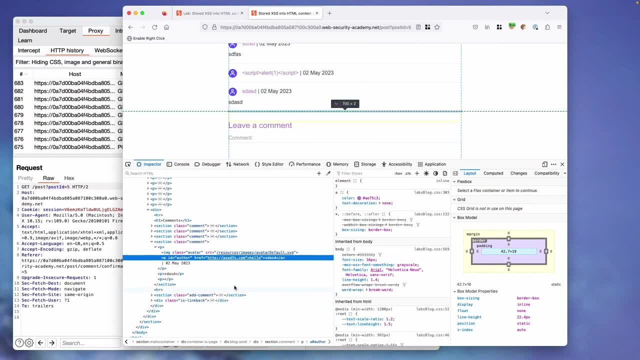 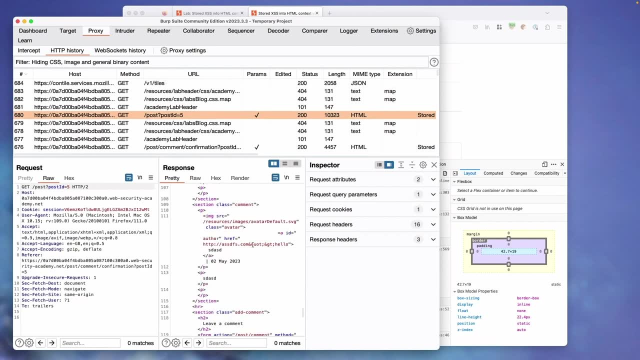 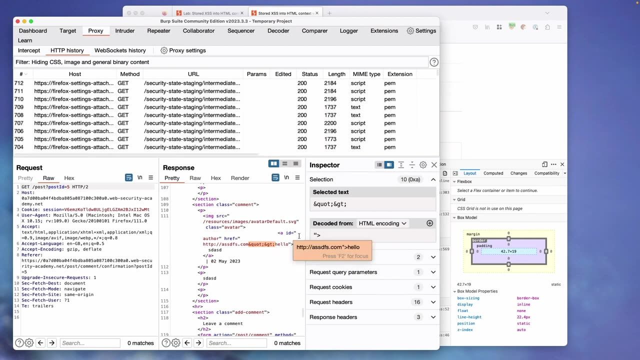 no, okay, try this. does it work? no, and here we can see that if we have a look at the request again, another response- we can see that once again, this is being computed as a quote and then a greater than it's not. it's being encoded as the.